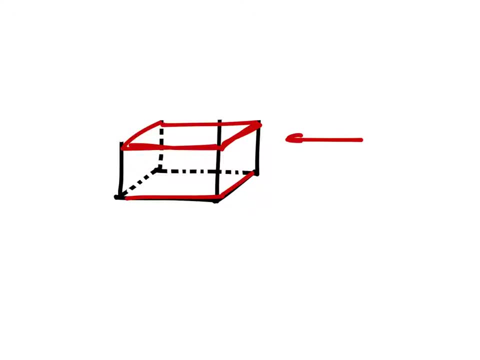 we look at that red piece right there. what? what shape is that red piece? A cube? Yeah, since this is a cube, if we were to move this so that we could see its face, oh, that's not very good, but it would be a square, All right. so that cross section. 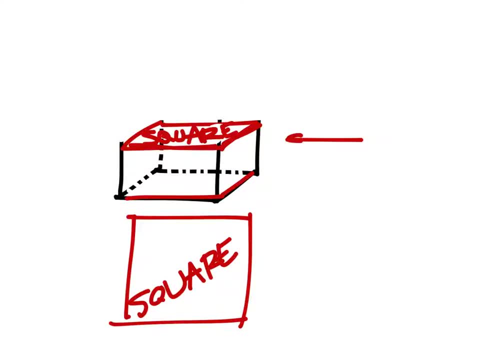 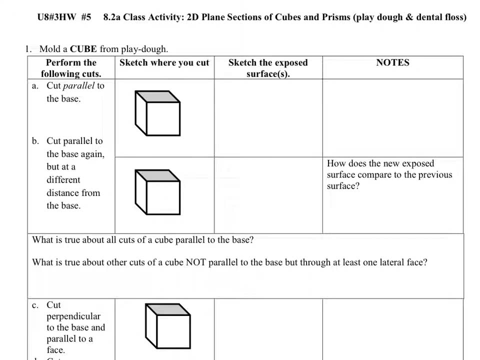 gives us a square Right here. All right, this next one. we want this cut parallel to the base again, but at a different distance from the base. So let's go ahead and sketch. we'll sketch the exposed surface as well, But let's go ahead and chop it somewhere else. 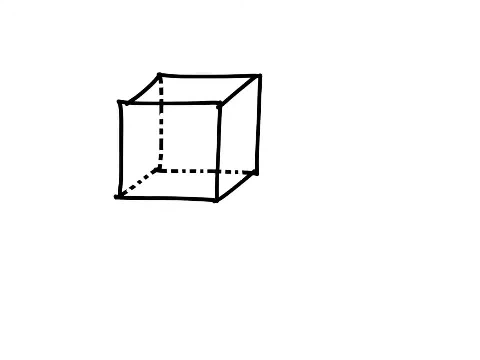 So this is the shape that we have Before. we cut it pretty much right in the center, right here. we're going to take that back and move it upwards right here. Now again, I'm just cutting this straight and horizontally right here. So now, if I cut this off like, 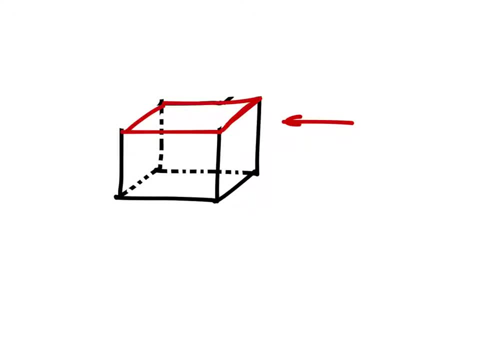 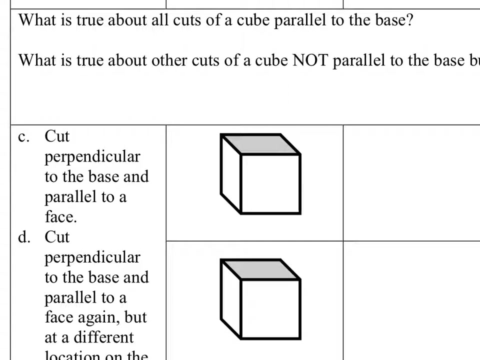 this. Then what shape does we have? Square, Yeah, still a square. So you'd still end up with a nice square-shaped red cheek. So what is true about all cuts of a cube parallel to the base they'll always give. 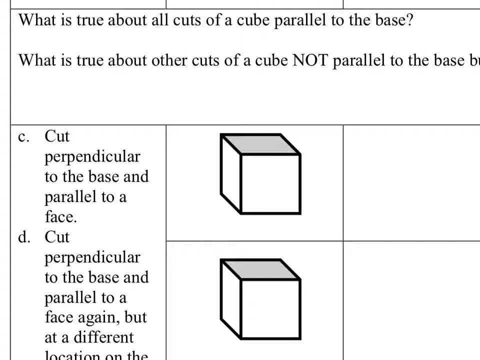 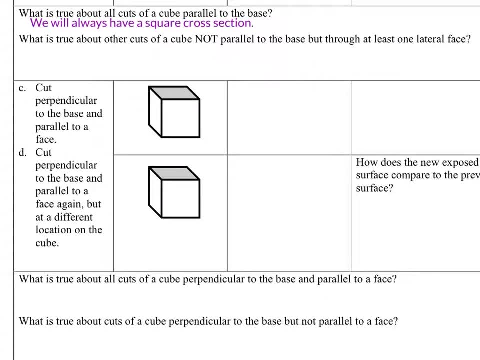 us squares. There we go. So the second part. what is true about other cuts of a cube, not parallel to the base, but through at least one lateral face? Again, these will always give us squares as well. Alright, let's move on to this next one. We're going to cut this one perpendicular to the base. 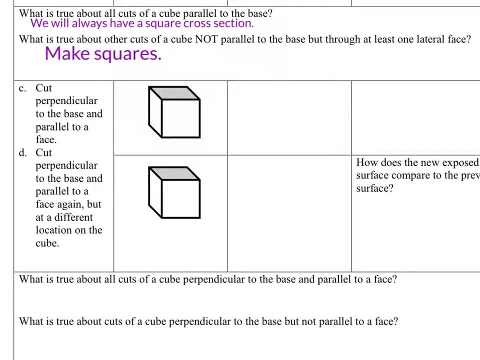 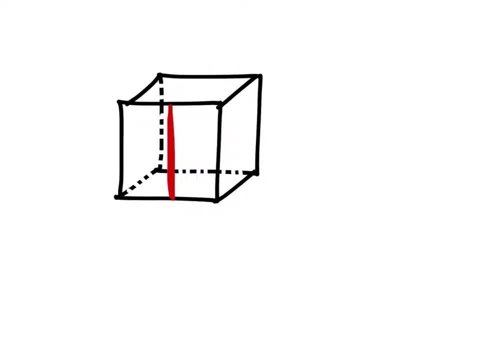 and parallel to a face. So on this one, perpendicular to the base means it's going to make a ninety degree angle right here. That's going to make it perpendicular to the base, but also it would be parallel, perhaps, to this face right here. So when we finish this chop, 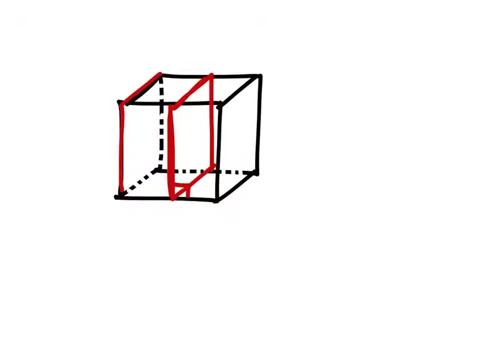 then we end up with something like these: Let's go ahead and clean that up. This is still a square If we move it out here. I mean, it's not very well drawn, but it is supposed to be a square. So, yeah, this would still give us a square. 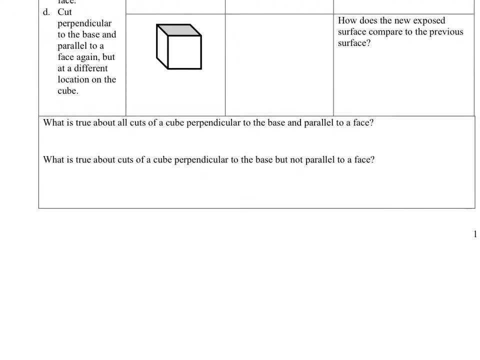 Then this next one: we're going to cut this perpendicular to the base and parallel to a face again, but at a different location. Is that going to change anything, you guys? No, If we did that, I mean, instead of cutting it right there in the middle, like we did? 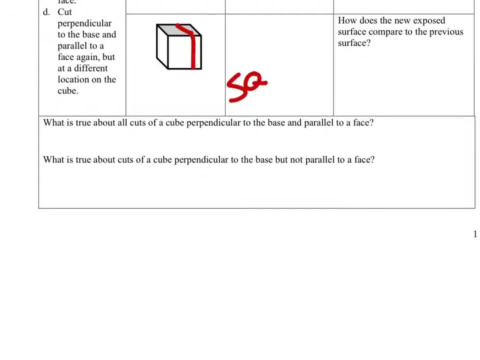 maybe cut it closer to the edge? yeah, that still will produce a square. How does the new exposed surface compare to the previous surface? They're exactly the same. Why, Right there Where Where we choose to cut a cube, as long as we're cutting it parallel to a face, then? 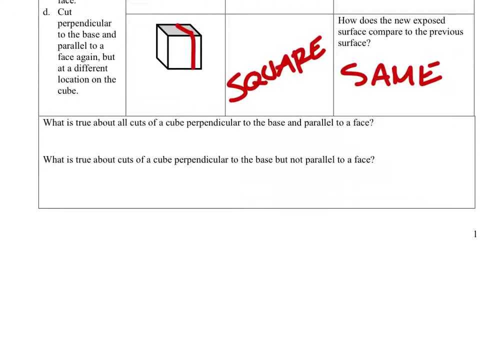 it will always be a square. So what is true about all cuts of a cube perpendicular to the base and parallel to a face? Always a square. What is true about cuts of a cube perpendicular to the base but not parallel to a face In a cube? if it's perpendicular to the base, then it will automatically be parallel to. 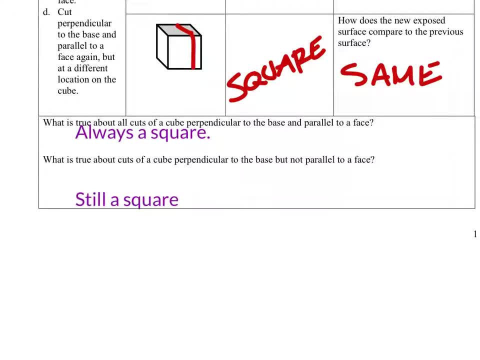 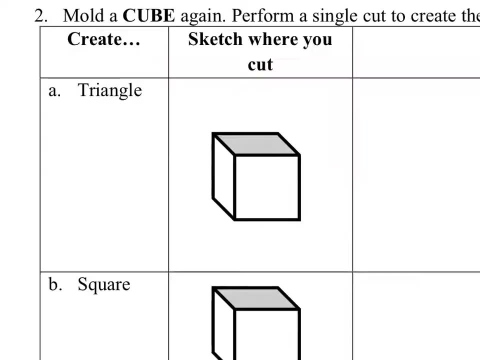 a face. So that's still going to be a square, Alright. so on these ones, we're just looking to see if we can cut this thing up to create different cross sections, different types of cross sections. In this one, we are going to cut this up to make a triangle. 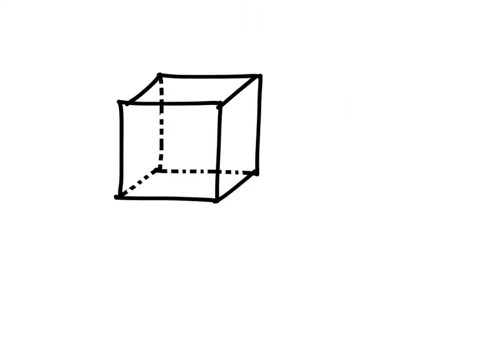 And then we'll move on to the square in the other ones. Alright, so I need a triangular face. There's several ways that we can do this, depending on the size of the triangle that we want. First up, what I can do is if I cut this thing. let's say I cut this through a diagonal of. 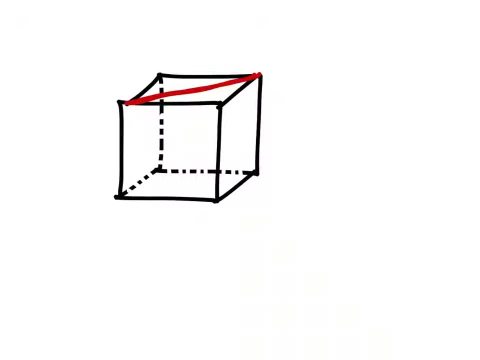 one of the squares. and now what I'm going to do is I'm going to cut this diagonally through to this corner right here. What that will do is I'm going to create a triangle like these, and then these other pieces kind of just go. 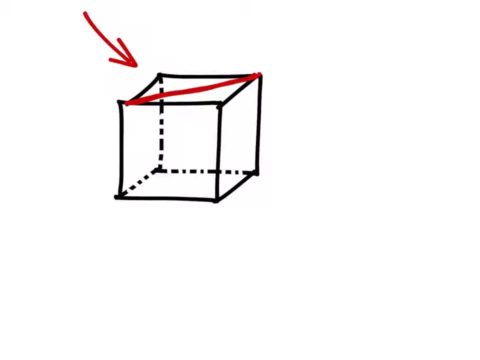 away. So I started by placing the knife here across the diagonal and then I sliced it straight down into this corner to create this triangle right here. Now this is what we did, is we started right there, but if, for some reason, we wanted a smaller, 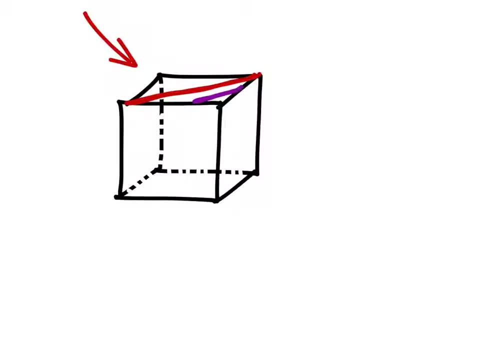 triangle. all I would do is place the blade farther to the corner, but I would still slice it diagonally against this corner, and then that creates a little triangle, radical. So it depends on the size you want on this, alright, But that would give us a triangle as well, just on that little corner of that cube. 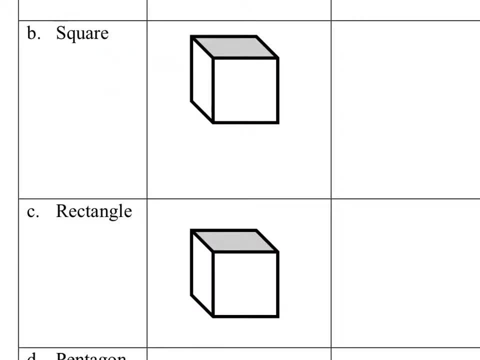 What about a square? Why don't we cut this thing to make a square? Yeah, we did it. You could cut it this way and then cut it straight back. That's going to make a square. Or you could cut it straight back like this if you wanted to. 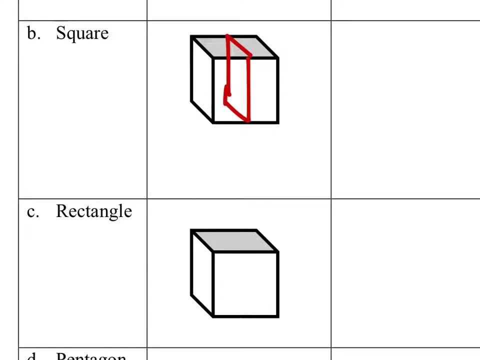 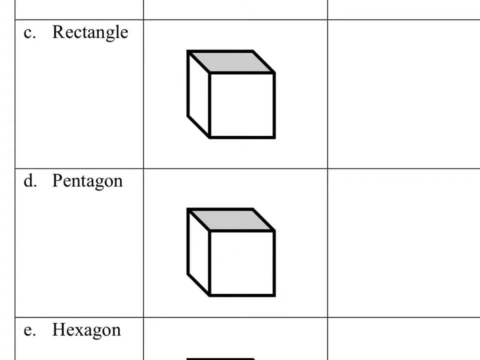 Either of those would give you a square- Alright. A rectangle, Alright. A rectangle is close to the square and we- just all we got to do to make this a rectangle- is to take what would have been a horizontal slice, like these, and, instead of cutting it, 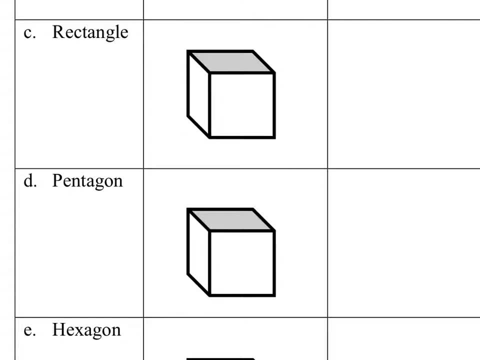 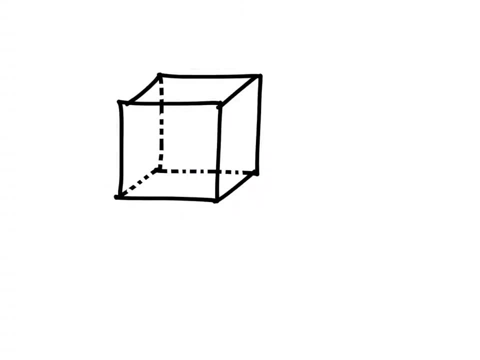 straight, horizontally parallel to the base. all we've got to do is angle this thing. So, instead of cutting it that way, I'm just going to angle it like these. Actually, we'll look at this one, So I'm going to cut this angled right here. 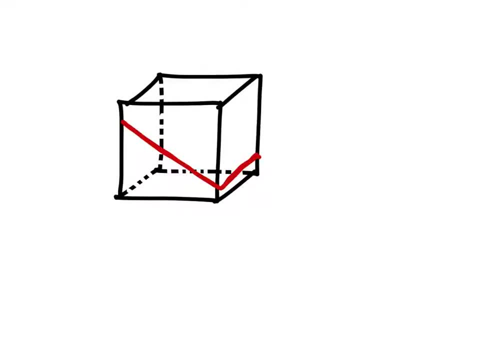 So what that's going to do is it's going to cut straight back onto these and this. Now we can see that this side is longer than this side right here. Let's go ahead and clean that up, Alright. now what happens is we've got these two lines and they are parallel to each other. 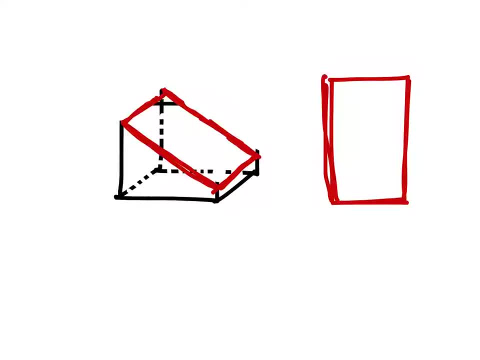 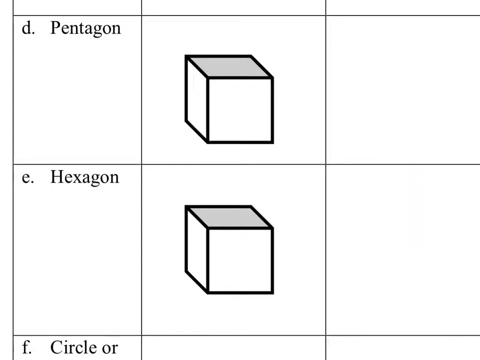 but these edges now are elongated to make this now just a rectangle And not a square. Alright, next we need to make a pentagon. So you guys take a moment and see if you can do that. If you can do the pentagon, then try the hexagon thing. 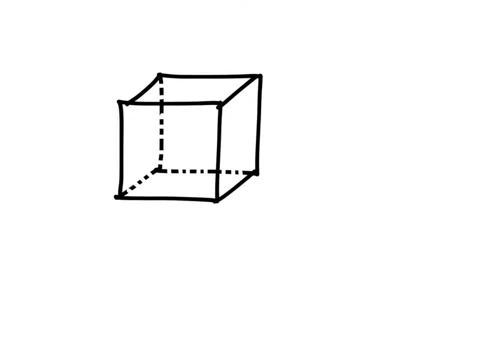 Jump it up so that we've got a pentagon, but we can only afford to make one slice. Now here's the problem is, if you make two slices, then you've got more like a three dimensional shape anyways. okay, So it's got to be one slice and one slice only. 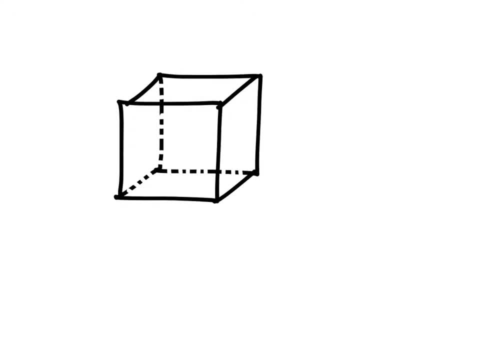 Here we go. What I will do is I set a pentagon first. A pentagon has five sides, So something that would be kind of like a regular pentagon looks like these. So I need a shape that looks like this. It may be elongated by the time I finish, because I'm not perfect at slicing. 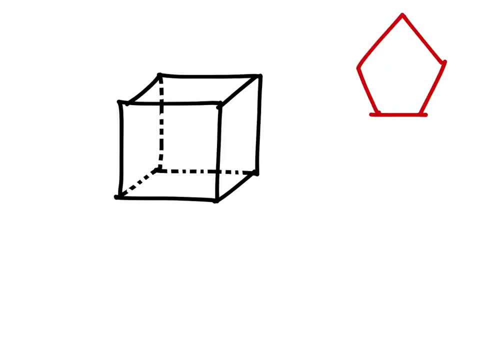 But I should be able to get this done. Here we go. What I'm going to do is I'm going to take the blade and I'm going to place it right here, but I'm going to slice this thing at an angle right here. 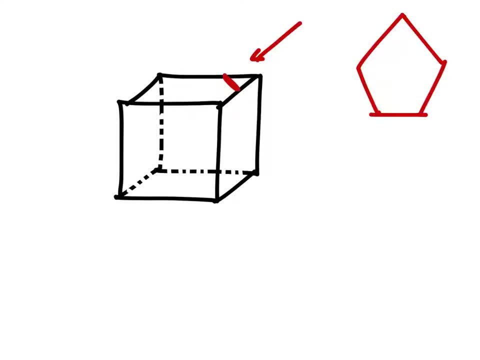 Okay, Alright, Now some of you guys see what will happen, But I'm going to make it so that it comes down to this point right here, Okay, So what's going to happen as I slice downwards or diagonally, is it's going to make these. 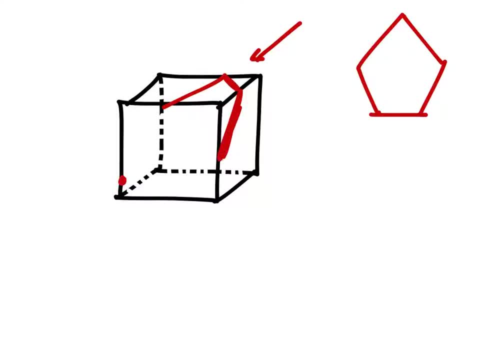 two lines right here, something like this, and then they will come into that point right here. Let's go ahead and clean this up so you guys can see what the heck just happened. Bam, There, it is This, This, This: 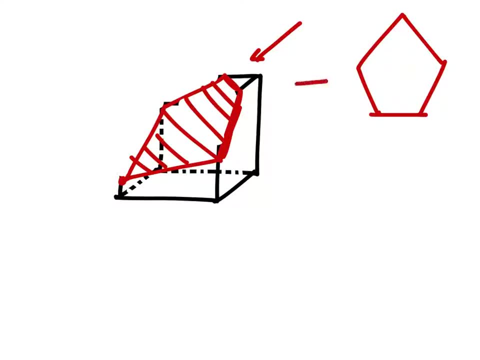 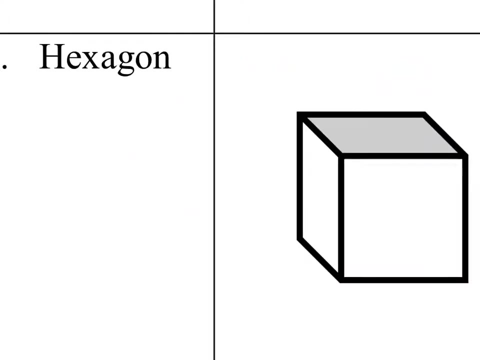 This, This, This is a pentagon. Now, this one is kind of sliced upside down. right, It will look something like this Mine's, sliced kind of upside down, But it is, It's a pentagon. All right, next up we will make a hexagon. 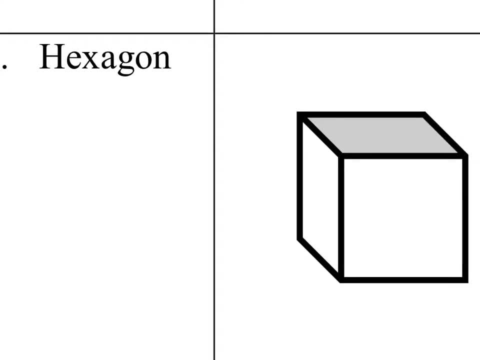 By making one cross-section or one slice into this cube, And this will be a hexagon because there's an X, and so I'm going to clear this. this cube, This one is really fun. Alright, this one. I made this a little bit bigger. 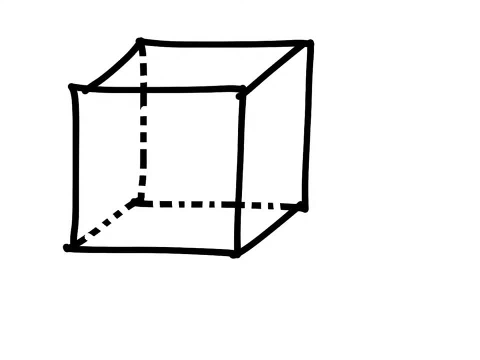 so we can see this. So some of you guys noticed, on that last one, when we cut up this thing to make the pentagon, we started about right here and then we sliced diagonally into this point right here. Well, that made a pentagon. All I want to do now is slice it so that when 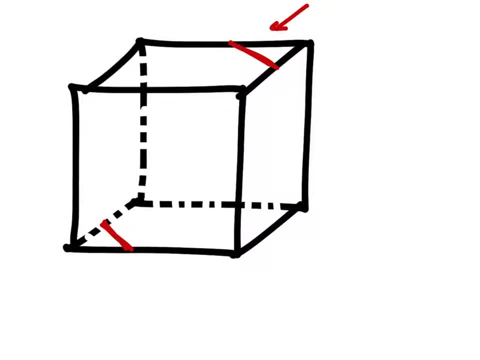 I end my slice, I'm going to end up on the base right here. So what will happen is I slice downward and it's going to come to this corner, and then it will come to this corner On the other side. it would look something like these, And this has six sides. now Let's 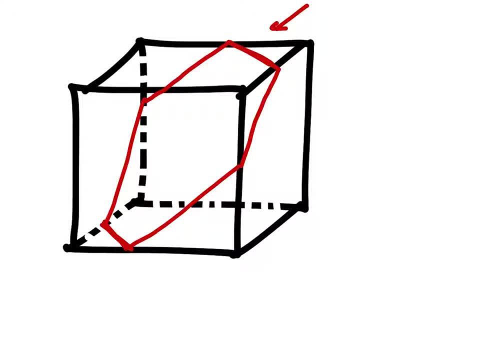 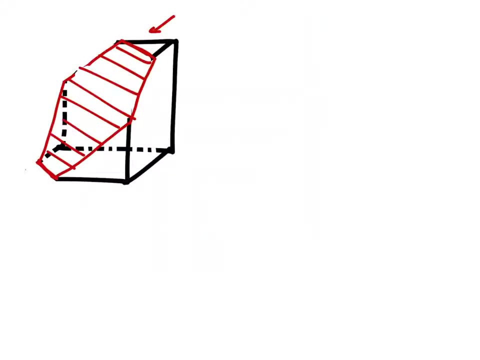 go ahead and clean this garbage up. Bam, We did it. Now we'll just shade this in so we can see this hexagon. Let's go and draw it on the side as well. Alright, let's go ahead and draw this to the side now. So 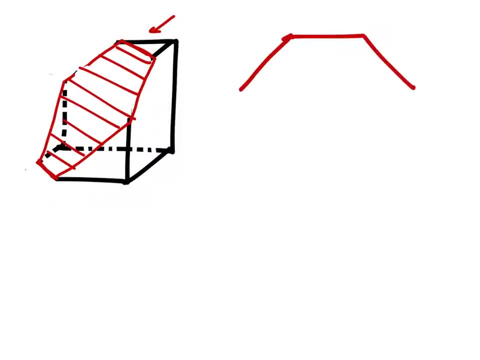 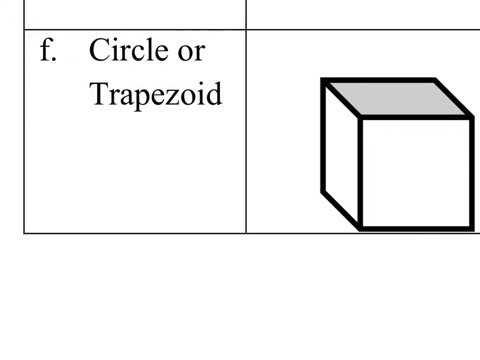 we got the straight line. We got this portion right here. I guess it's kind of elongated right there, but that's still a six-sided hexagonal shape. Alright, can we make a circle or a trapezoid with a cube? Um, we certainly couldn't do. 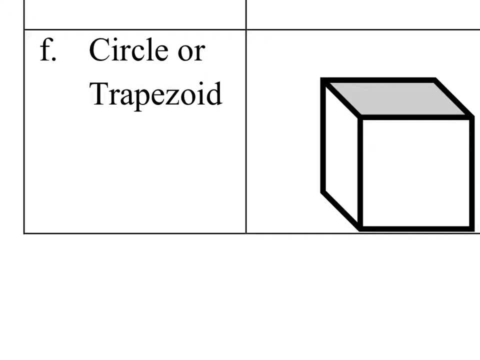 a soycle, because there's no way to get a soycle out of this with one cut. That is just a cross section. You can't do the circle, That's not going to be possible. I can make a trapezoid out of this thing though. 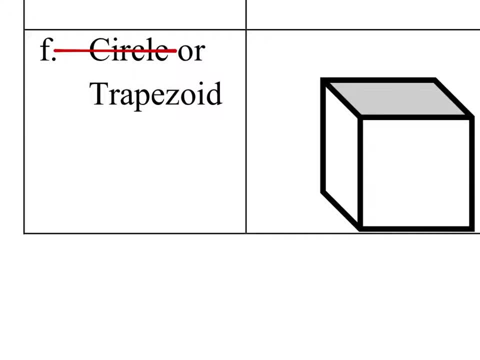 The thing that I'm going to do is I'm going to make a trapezoid. I'm going to make a trapezoid. The thing that's unique about a trapezoid is that it has one set of parallel sides. 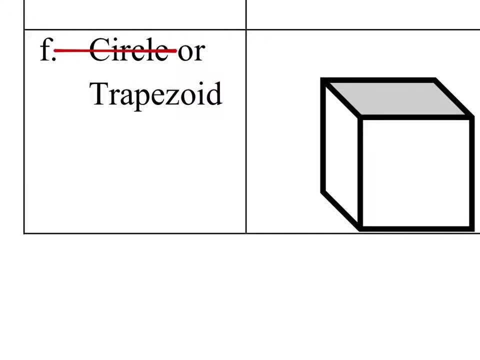 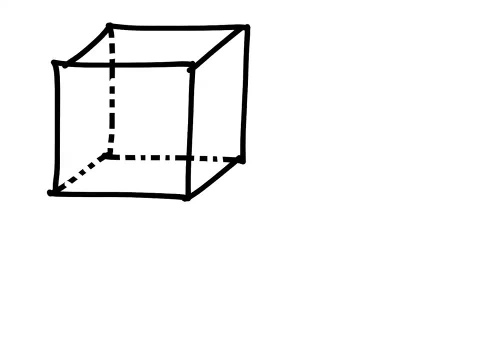 and the other two sides are not parallel. If they were, then it would be a parallelogram. So let's look at cutting this up into a trapezoid. Alright, so let's take this shape So to make the trapezoid. what I'm going to do is I'm going to start my slice right here. I'm going. 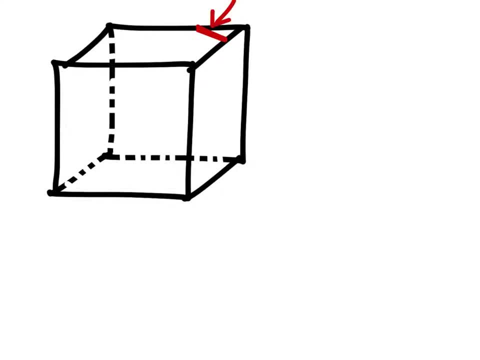 to go diagonally, but I'm going to change the angle on this so that it doesn't reach these corners right here. So what that means is I can get down to this diagonal right here. So what happens when I do that is it creates a shape like these. Let's clean that up And 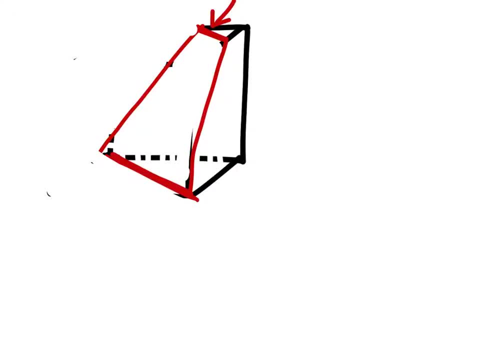 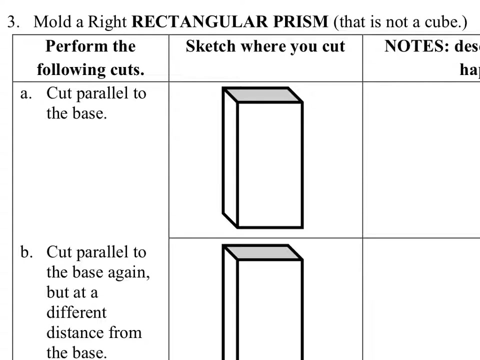 yes, right here we've created a trapezoid. If we drew it separately, it would look something like this, Something like this, where these two side lengths are parallel: The right rectangular prism- that is not a cube, which we're looking at right here- And the first one A. it says: 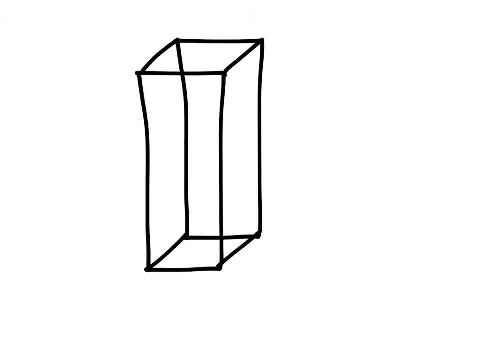 to cut parallel to the base. So the base on this one we're going to say is this bottom. we'll say it's a square right here And we're going to cut it parallel to the base, which means I will put a razor blade along this line and then I would cut straight horizontally. 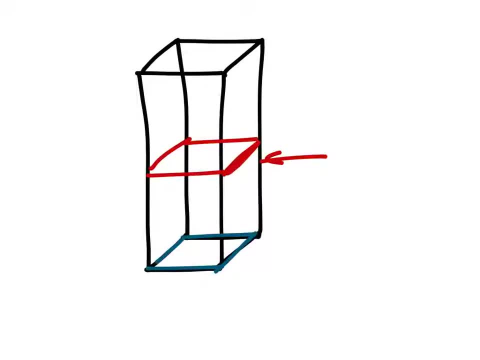 And now what has happened? Let's go ahead and clean this up, okay. Now here's the problem, and some of you guys are still saying: rectangular prism, The cross section, is not a three-dimensional shape. What shape did we create? 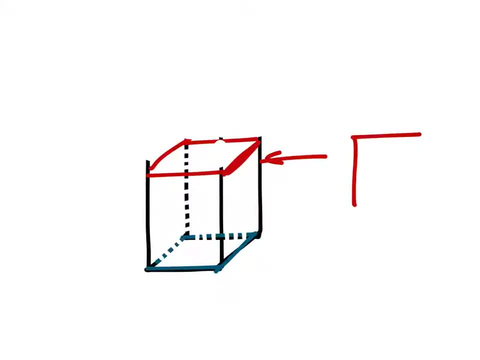 We're a square. Yeah, this one looks to be a square, A square bottom. Those sides are not even Well, they were supposed to be. if I'd used the other one, Yes, this would give us a square. If you said rectangle, that would be acceptable, unless they told us that the base was a square. 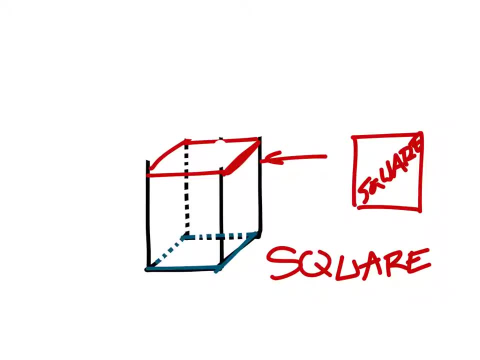 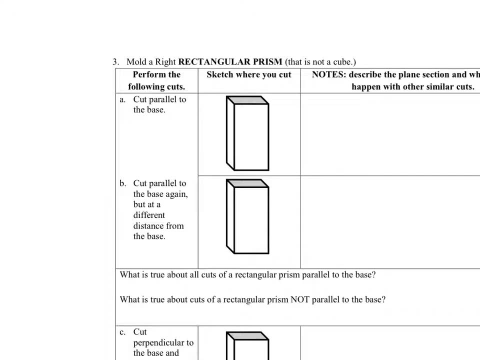 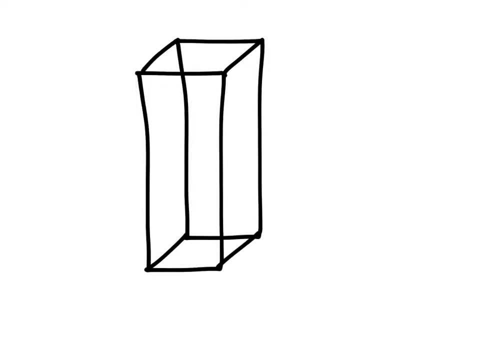 All right. this one says: cut parallel to the base again, but at a different distance from the base. All right, let's go ahead and do that. All right, so I'm going to last time. I cut it about right here You guys want me to be. 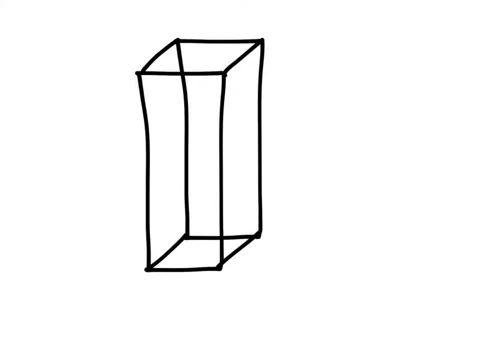 closer to the base or farther away, this time, Farther, Farther. okay, So I'm going to cut it, let's say, towards the top up in here, And this is going to be parallel, so I'm going to be cutting this straight horizontally. 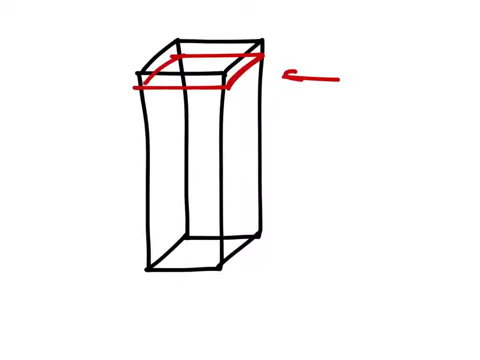 Exactly. So that would give me some kind of shape like these. Let's go ahead and clean it up. All right, so that gives us this cross section right here which, yes, appears that it would be a square. Now again, I'm okay if you put rectangle on this, because it didn't specify that base was. 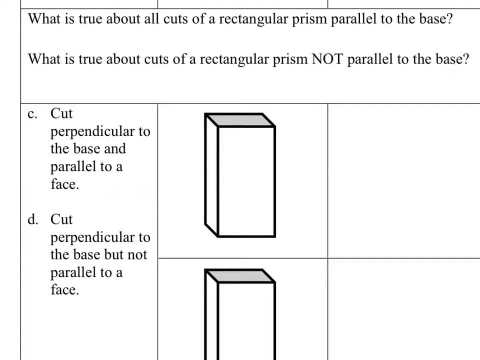 a square, All right. what is true about all cuts of a rectangular prism parallel to the base? Parallel, Parallel. So the cross section that we make would be the same shape as the base. Well, what is true about cuts of a rectangular prism not parallel to the base? Then it depends It. 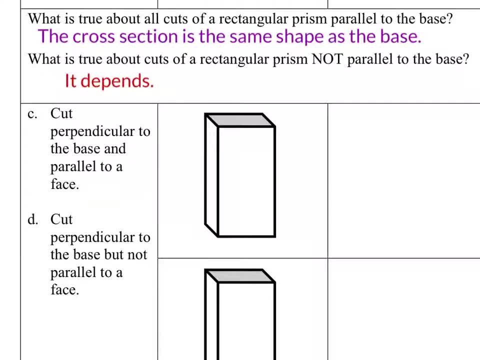 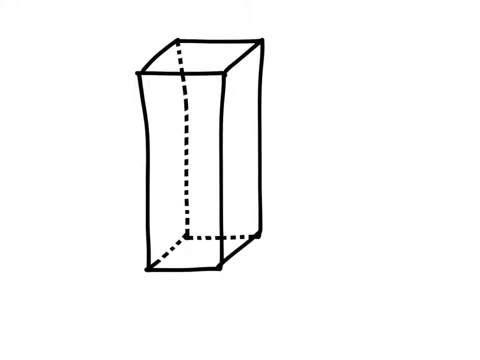 we do need to cut this perpendicular to the base. The base is that bottom shape for now, And so what we're going to do is perpendicular would be like placing the razor blade right here, which would make a 90 degree angle with the base. Now, when I do that, I'm going to 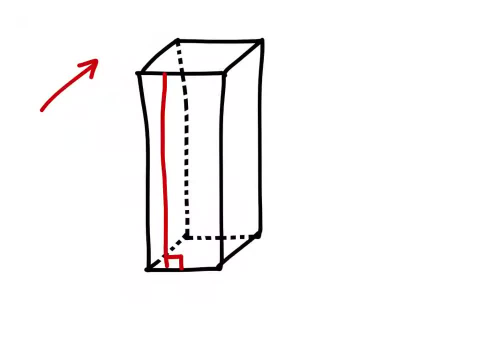 be just cutting straight back into the shape. So this is a horizontal slice which this shape right here Is going to be. let's go ahead and clean that one up as well. So again, we're looking at the cross section right here And, yes, that will create a rectangle you can call. 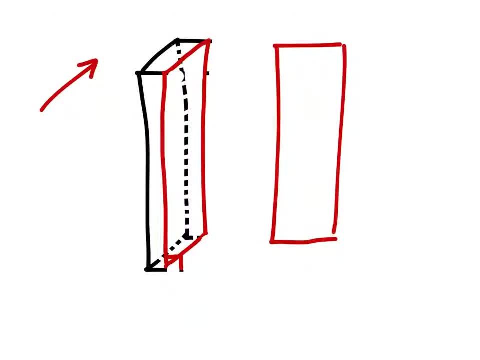 it long and skinny if you want, but it should look something like this: But that is definitely a rectangle. Oh yeah, so when it's said to cut it perpendicular, so we made that perpendicular to the base and we made it parallel to this. 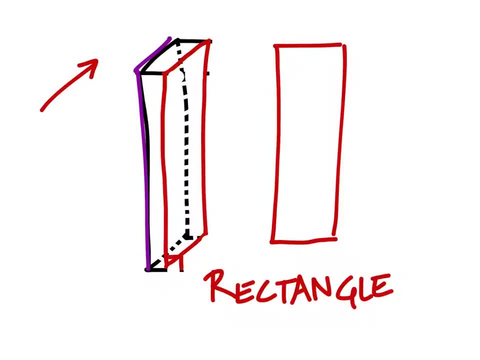 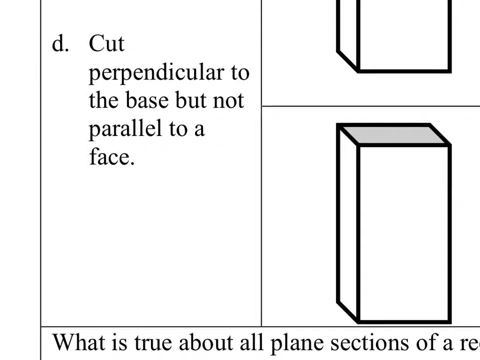 face here on the left. So that's what that meant by parallel to one of the faces. So we need to cut this perpendicular to the base but not parallel to a face. This one's a little confusing, because if we cut it perpendicular to a base, it'll be parallel to two. 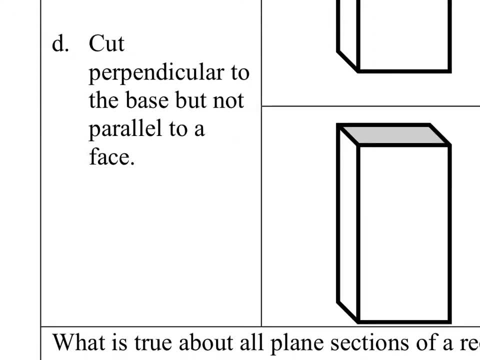 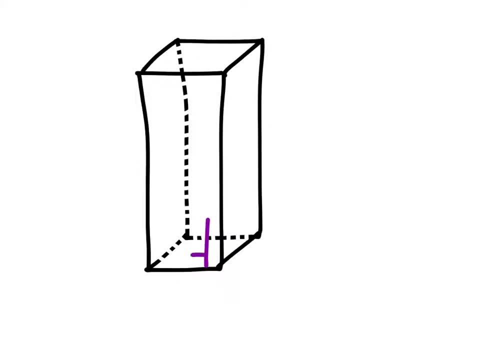 of the faces. So I mean we could make the same cut on this thing. So perpendicular to the base means it's going to create a 90 degree angle with the base. Now, in this case, I mean that's as far as we can go on. 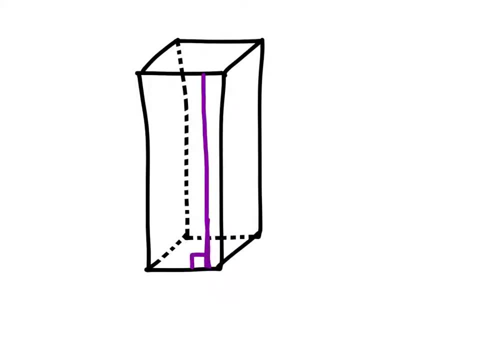 that thing. So we could say that it's not parallel with one of the front faces, But in any case, we see that it gives us the same shape, the rectangle. So that's our rectangle right there, And we can draw it separately as well. Something like this: 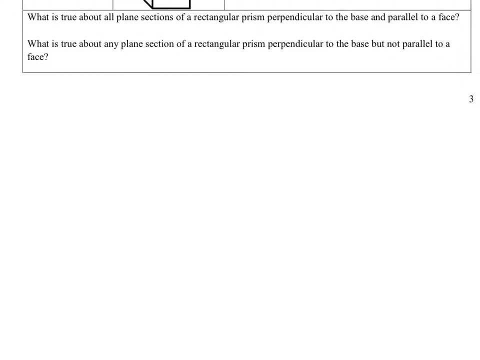 What is true about all plane sections of a rectangular prism? perpendicular to the base and parallel to a face? It will give us the shape that is cut, the parallel shape that it's cut with. Yeah, that sounds good. What is true about any plane section of a rectangular? 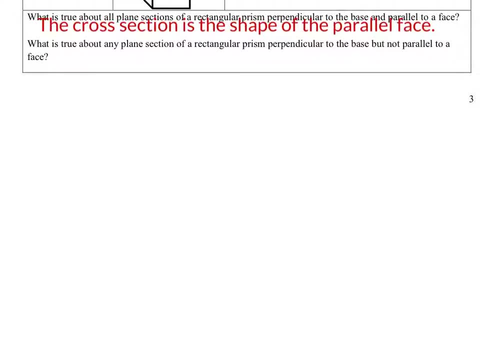 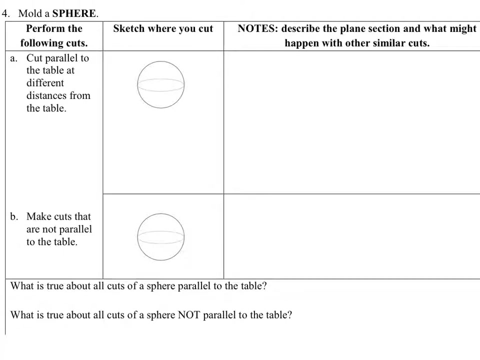 prism perpendicular to the base but not parallel to a face, Unexpected number of times. right Now we're looking at spheres And this first sphere, we're gonna cut it parallel to the table, at different distances from the table. So let's. 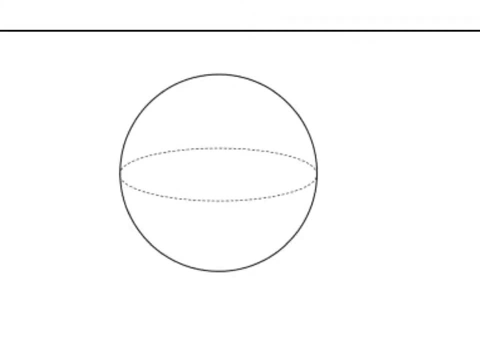 go ahead and do that. So, around the count, if I cut this thing, let's say that we cut it first right down the middle, because this would be sitting on a table right again. well then we would get this shape. that wasn't good, but yeah, now that's the. 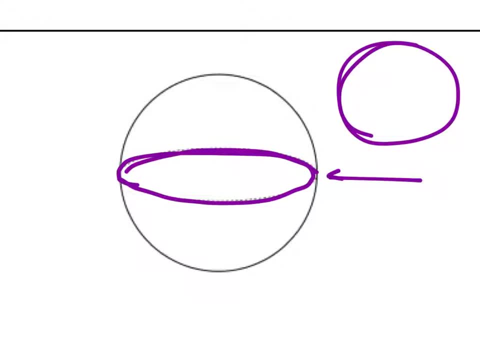 three-dimensional shape which, if we moved it to the top, we would see that this is a cycle. but what if I cut it at a different distance from the table? alright, so I'm cutting it right account, which also would make a circle, just a smaller one down at the bottom. so, as it turns out, no matter how far away you are, 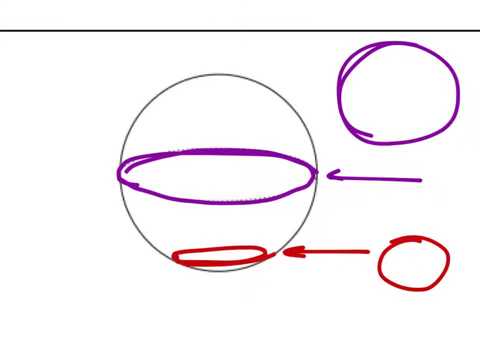 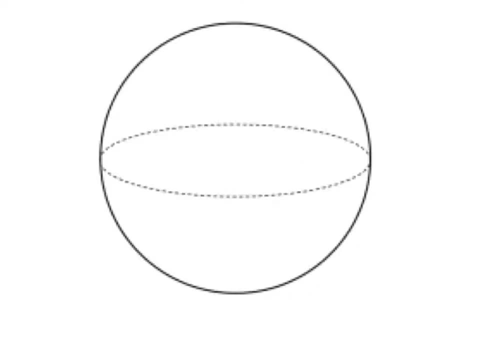 from the table. if you cutting it parallel to the table was, it will always be circle. alright, now let's make cuts that are not parallel to the table. all right, now here's the thing is: if I cut it straight down, right account at the top it'll. 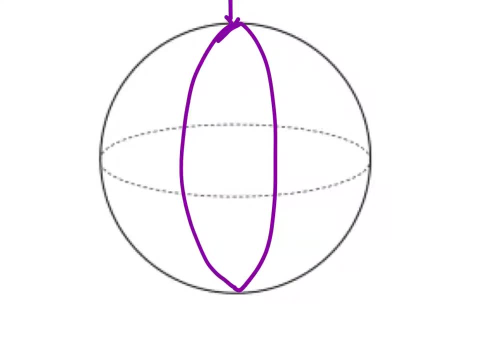 still be a circle. right, we just change the orientation of the circle. But what if I cut it diagonally? This is still going to end up being a soil radical. So what if I cut it down diagonally? this way, It's still going to give you a soil radical. 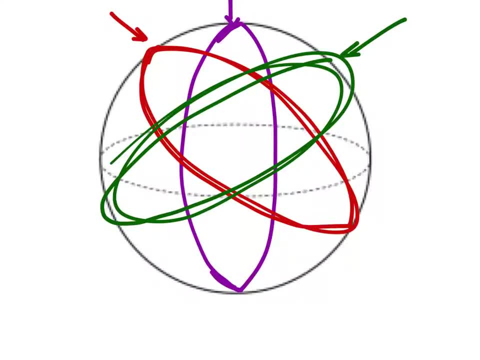 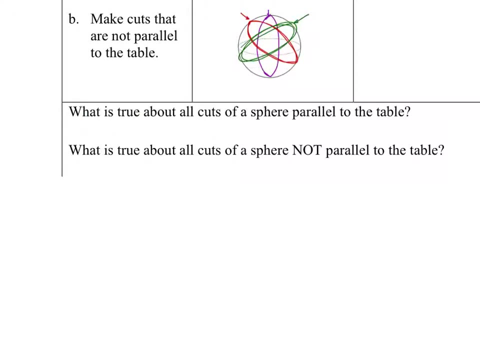 And, as it turns out, it doesn't matter where we cut the soil radical. we will always get some type of soil radical. What is true about all cuts of a sphere parallel to the table? They're all circles. And what is true about all cuts of a 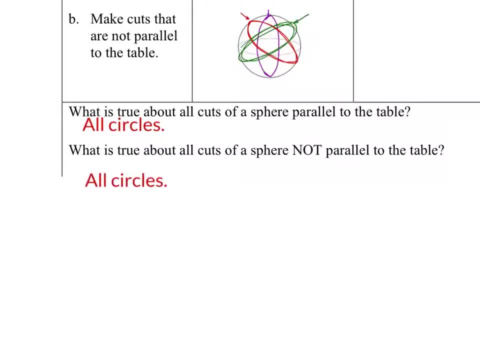 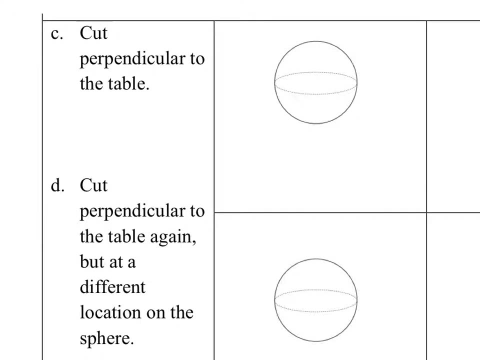 sphere, not parallel to the table, Still circles. Now, we did cut. we did make a cut perpendicular to the table already, So let's make this first cut perpendicular to the table. So again, if the table is on the bottom, we're going to cut it straight up. 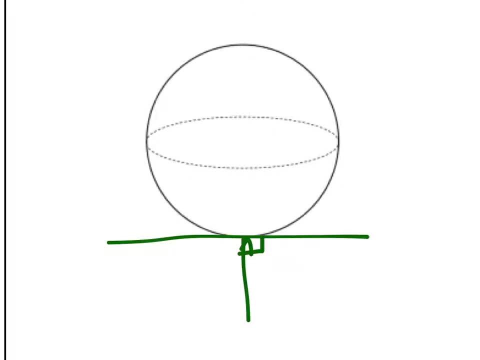 creating a 90 degree angle radical, And that would give us still a soil radical, Something like this. Now, this does look like an oval because of the 3D shape. However, if we took the 3D shape apart and then showed you just the two-dimensional face, 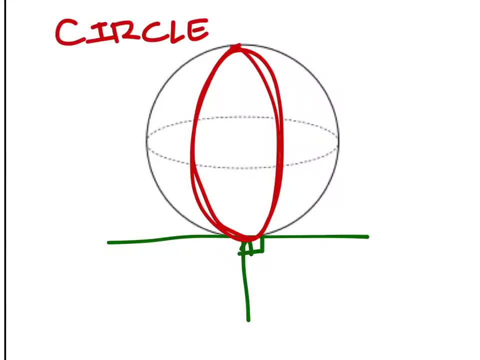 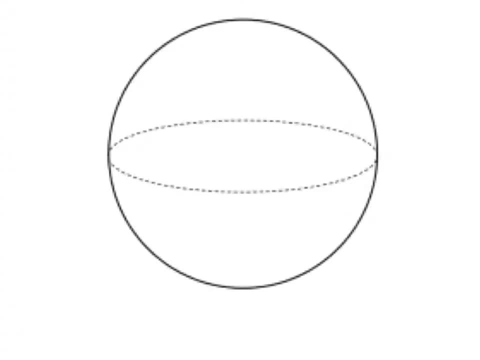 it would be a circle That's cut perpendicular to the table again, but at a different location on the sphere. So still perpendicular. I'm going to cut it straight across. radical. And that's going to be a circle. it's just a smaller circle, radical. 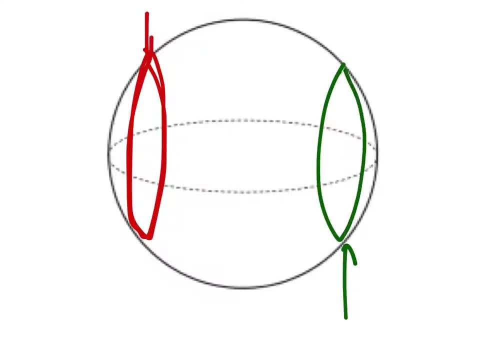 Same. if I cut it all the way down It would be a circle, but again it's just smaller. I mean, I could cut it here and it would still be just now, a bigger circle maybe. So what is true about all cuts of a sphere? 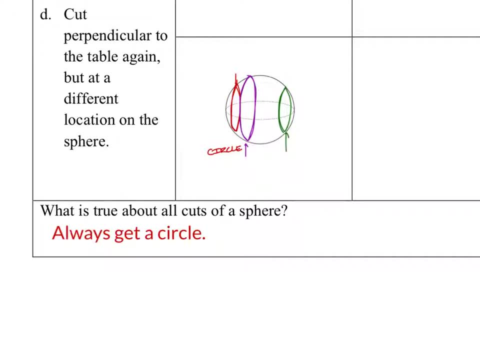 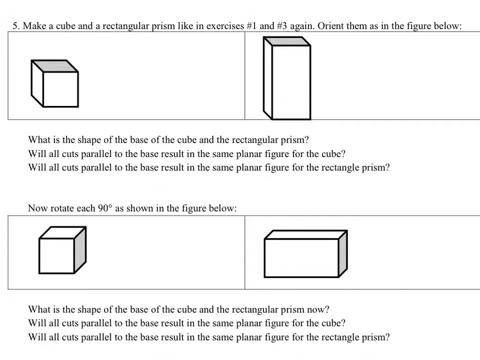 You always get a circle, Make a cube and rectangular prism. we have those. What is the shape of the base of the cube and the rectangular prism? Will all cuts parallel to the base result in the same planar figure for the cube? Yes, Will all cuts parallel to the base result in the same planar figure? 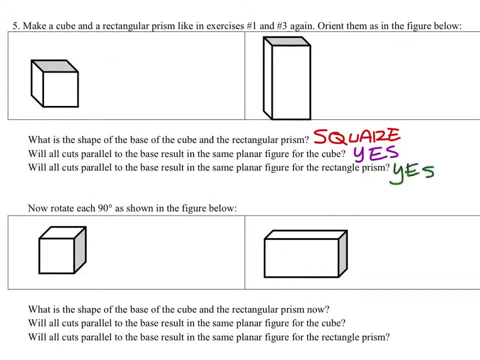 figure for the rectangular prism. So next up, we're going to rotate these 90 degrees each, which means we're just going to flip them over this way, which is why they're shown in the next two figures right around the count. So what about now, Now that we've rotated? 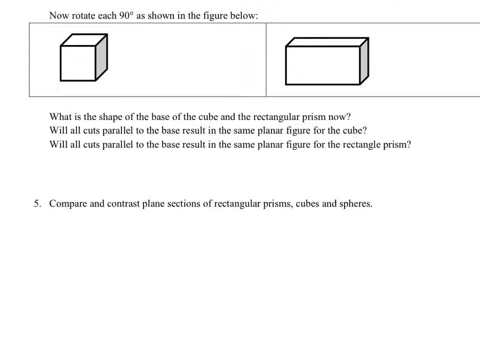 these. well, what is the shape of the base of the cube in the rectangular prism? now, Some type of rectangle. So that's a good question. Would it be a square and a rectangle? That is an acceptable answer. However, squares are types of rectangles, so I'm okay, just. 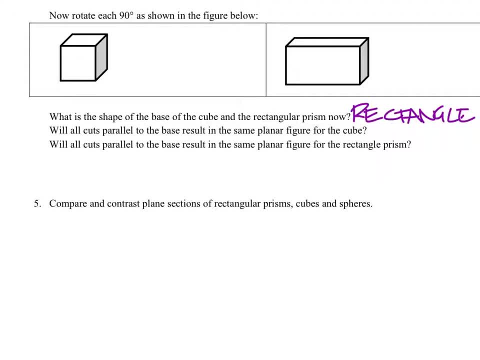 writing rectangle on this part. Will all cuts parallel to the base result in the same planar figure for the cube? Yes, they will. Will all cuts parallel to the base result in the same planar figure for the rectangular prism? That also is still a yes. You get rectangles right there. So compare and contrast planar. 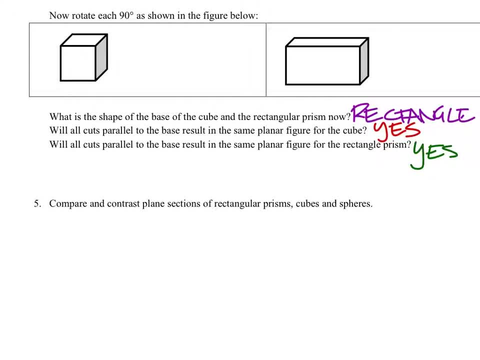 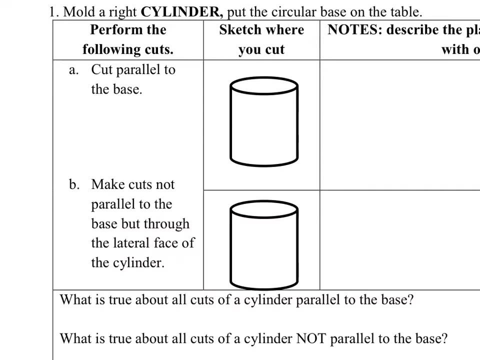 sections of rectangular prisms, cubes and spheres. All right, that seems like a pretty acceptable explanation of that stuff. So we're going to take the cylinder, The first one. we're just going to cut it parallel to the base and we'll see what cross-section this gives us. All right, so this says we've. 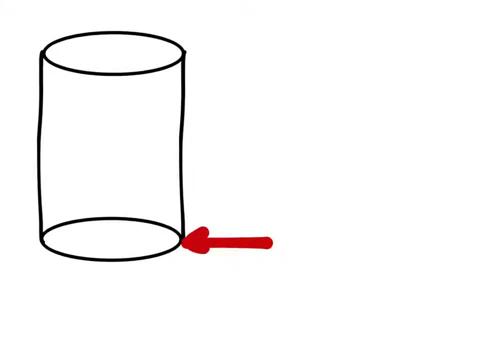 got to cut it parallel to the base. The base is kind of horizontal radical, So what we're going to do is cut a horizontal cut on these. So when we do that, what's going to happen is it's going to – that's not great, but 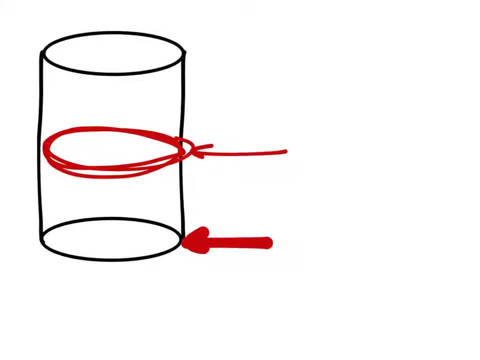 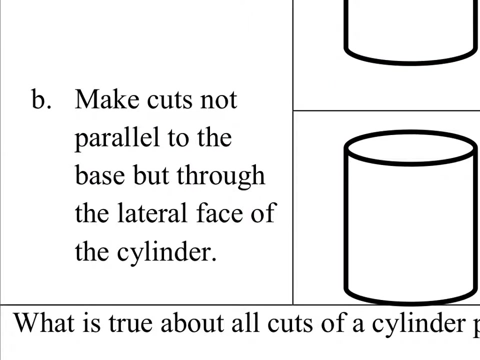 it works If I cut this off and let's clean this up. well then, what we get is this red shape which, if we looked at it straight, it would give us a circle like these. All right, the next part is to make cuts, not parallel to the base, but through the lateral. 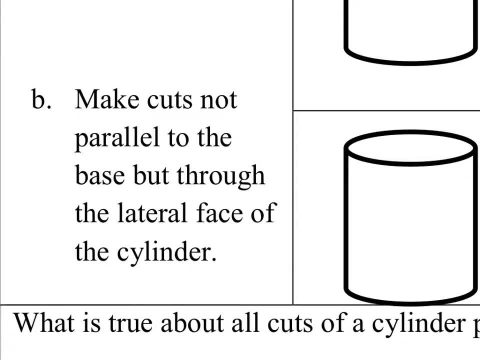 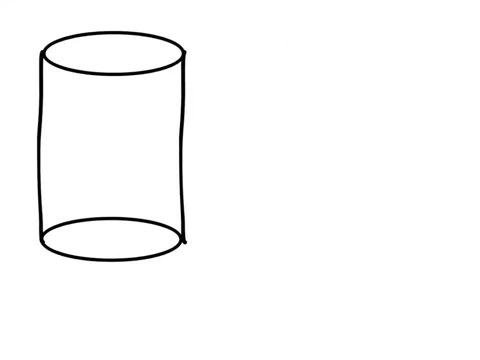 face of the cylinder. Here we go. Now. there's lots of different shapes we can make about this, actually, but let's look All right. so not parallel means that we've got to slant this thing just a little bit at least. So if I cut this at some kind of angle now – in 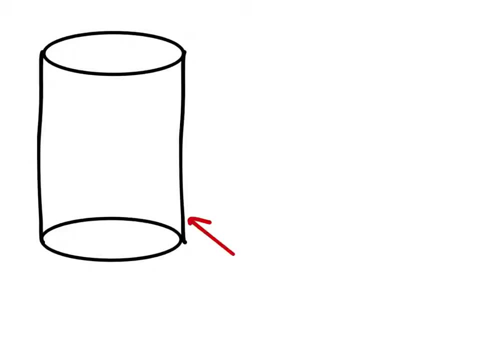 fact, let me exaggerate that even a little bit more- I'm going to cut it like these. So I'm going to start at this point with my razor blade and cut it all the way to the top, up and down. So if we look at these, it should look something like these, something like that. Now, if we 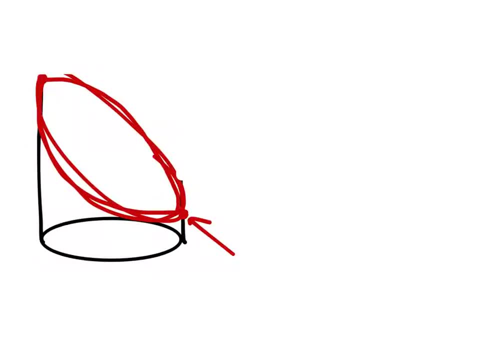 look at this shape – let's go ahead and clean that up. This would actually, if we looked at this straight on, this would be some kind of – you guys would call it an oval, maybe It's an ellipse, But yes, in math we would call it an ellipse. 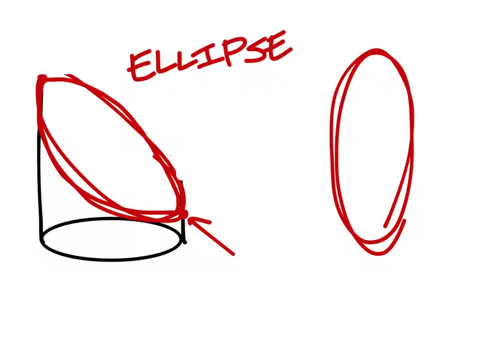 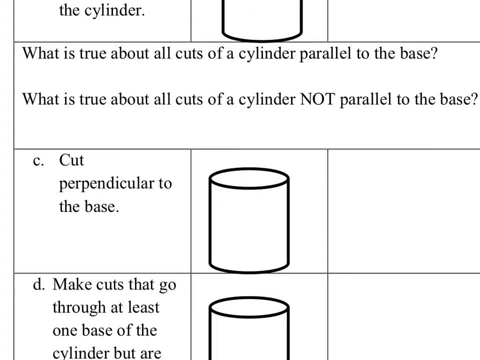 Can we just call it an oval? Okay, Okay. So this next question: what is true about all cuts of a cylinder parallel to the base? Well, that would give us all cycles. Then, what is true about all cuts of a cylinder not parallel to the base? Those are all going to be ellipsoid. Bam, there we go, The next. 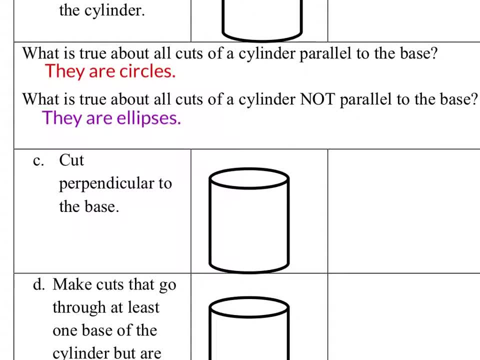 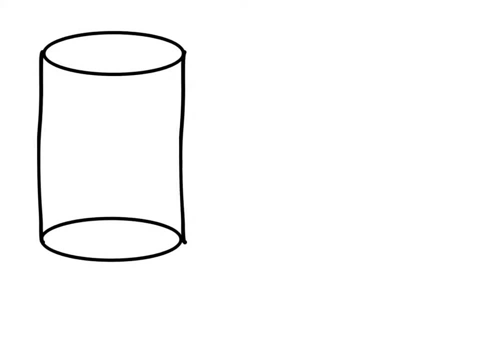 part is to cut this perpendicular to the base. All right, let's get that done. So perpendicular is at a 90-degree angle. So if this was the table, it would be at a 90-degree angle up and down. Now I'm going. 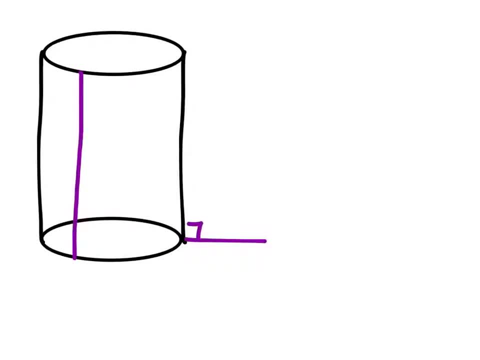 to actually be just placing the razor blade straight across. try to count, making a 90-degree angle with the bottom, And I'm going to cut this thing straight across through the middle up and down. So let's see what shape this gives us. Well, this appears to be some. 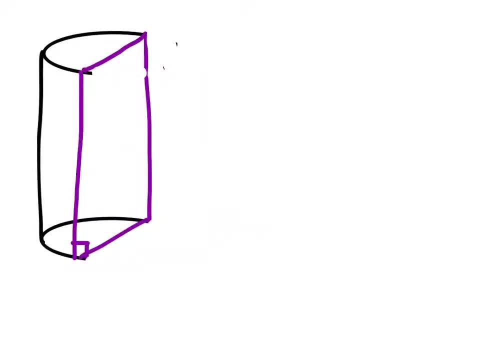 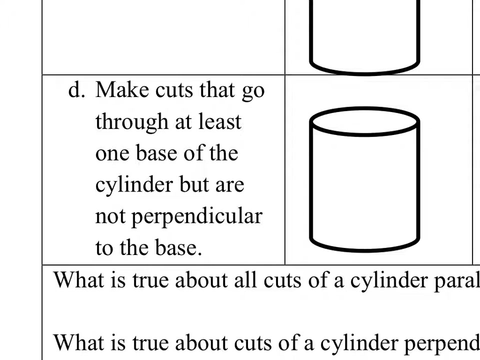 sort of rectangle. So let's clean it up, All right, and if this were a stamp of some sort – Then it would clearly be some kind of rectangle up in here. That'll do it. Yeah, nice. Part D: let's make cuts that go through at least one base of the cylinder, but are not. 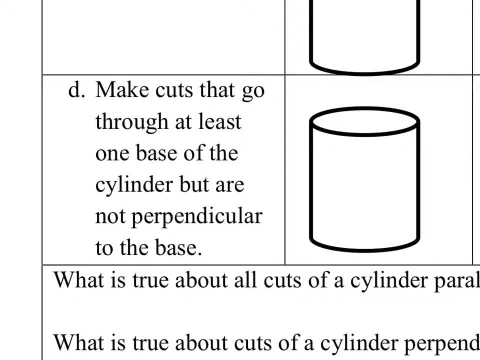 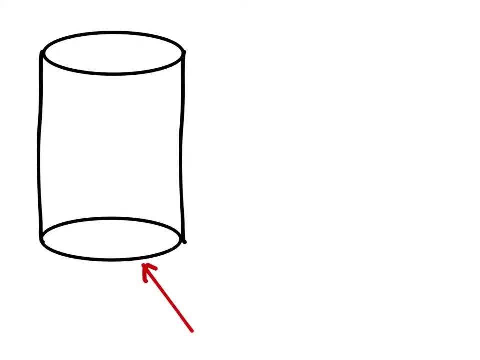 perpendicular to the base. So what that means is, when I'm cutting this, I'm going to cut through the base, but I'm going to be at some kind of angle up and down, So I'll start on this edge and I'll place. 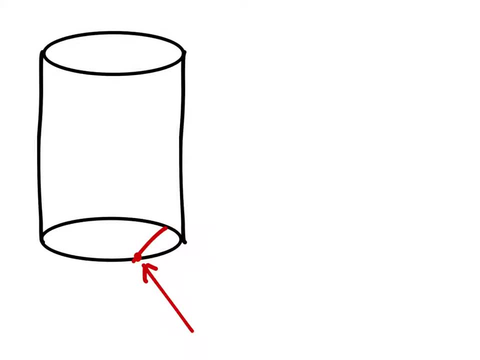 my razor, I guess, straight across if I want to. And yeah, if I went all the way to like the side all the way down, then it would create some kind of weird-looking part of an oval shape, Something like this maybe: 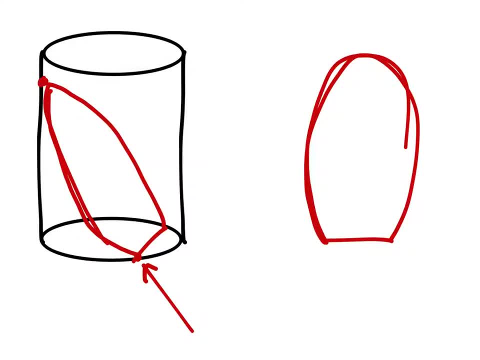 Now here's. the other thing, though, is, if I went all the way to the other edge, then it would be something more like this, So that'd be just with the edge cut off right there. 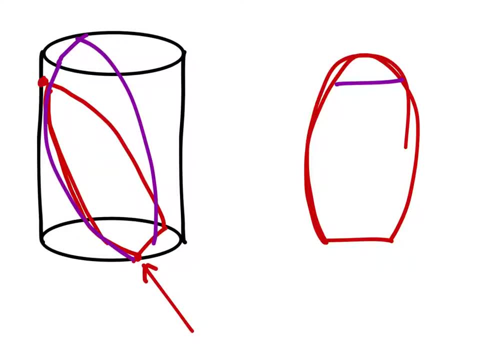 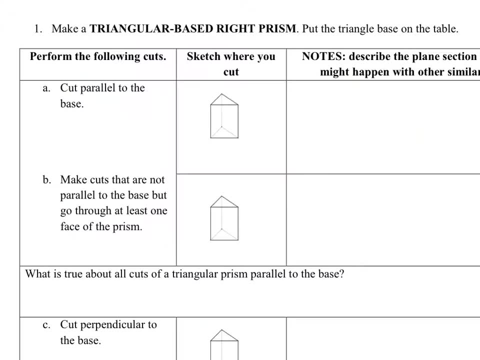 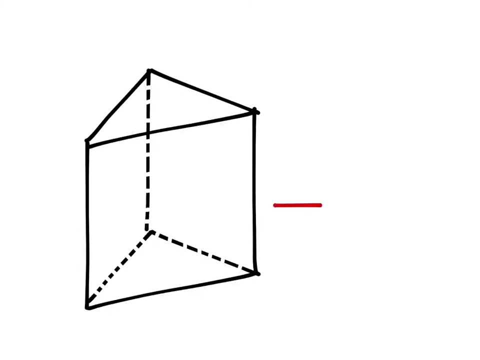 maybe. So it would be an ellipse with the ends cut off, or just one end cut off. So with these triangular-based right prisms, we're going to cut first, parallel to the base. 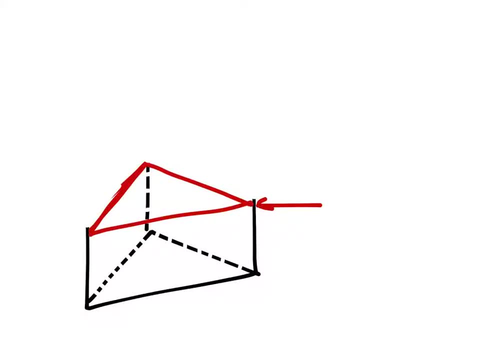 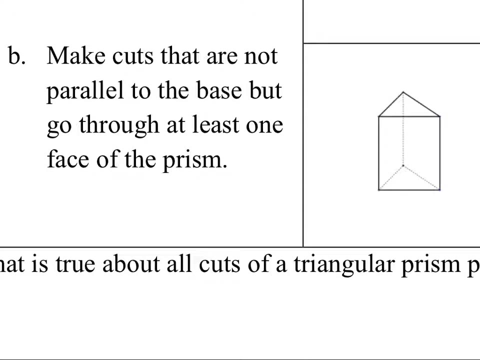 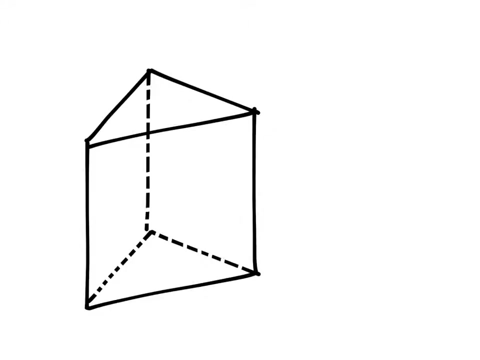 By cutting this parallel to the base Triangle. Well, let's go ahead and make cuts that are not parallel to the base, But go through at least one of the face of the prism, okay, So what I'll do Is just like on the last one: I'll still place my razor blade across the edge right now. 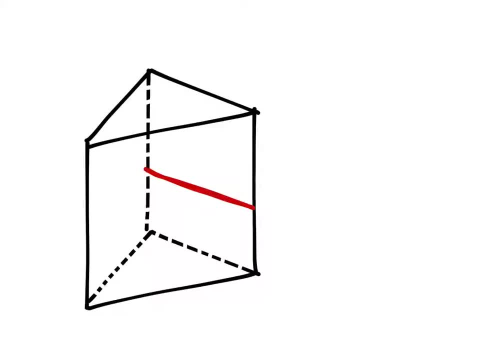 But there's a couple shapes that we could make. For example, if I went to this corner right now, Then I guess that didn't turn out very well. Let me go the other direction. I'm going to cut it down to this point at an angle. 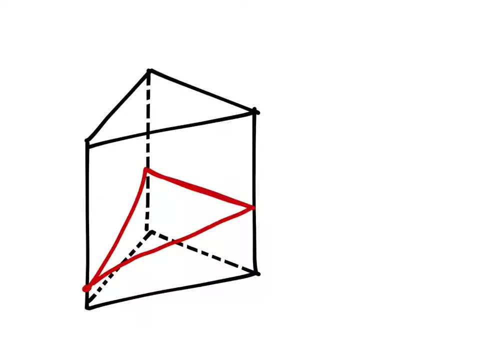 So this one is going to create again a triangle. But here's the thing is: if I went so that the blade would have cut through this edge right here, Or actually, let's, let's do it down right here- Well then the shape would have been a trapezoid. 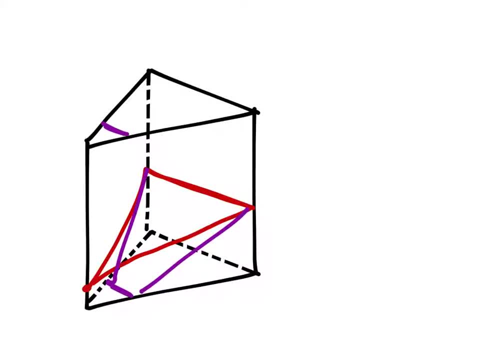 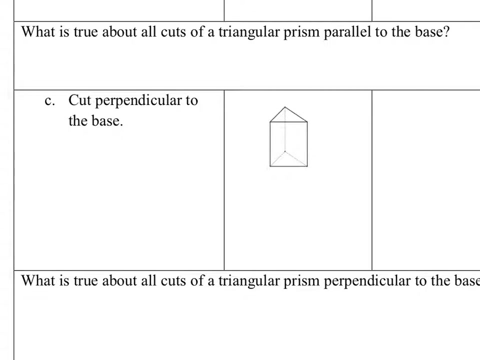 So we get two shapes possible. when we do not cut parallel to the base, Then it's got to be one of these two. What is true about all cuts of a triangular blade? The prism parallel to the base? Well, you'd always get a triangle. 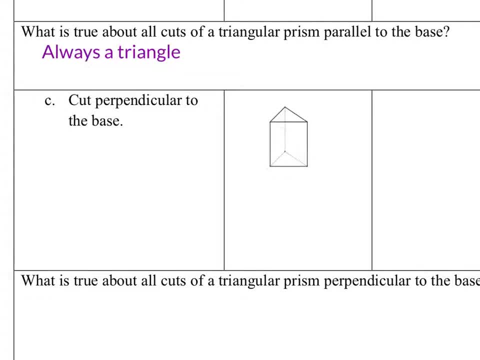 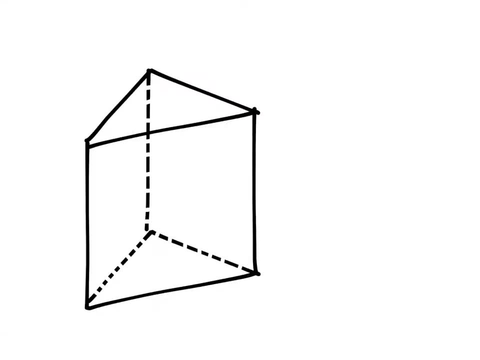 All right. next up, we're going to cut this thing perpendicular to the base. Yeah, that'll be good, All right. perpendicular means I'm going to place the blade of this thing straight up like these, making a 90 degree angle, and I can cut straight back on this thing. 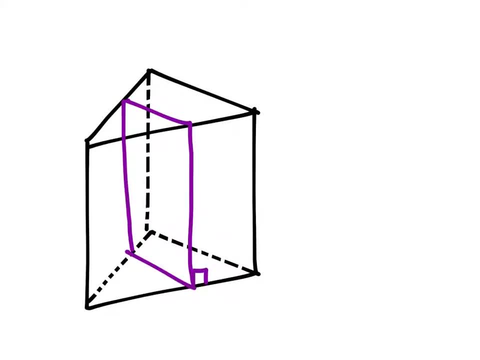 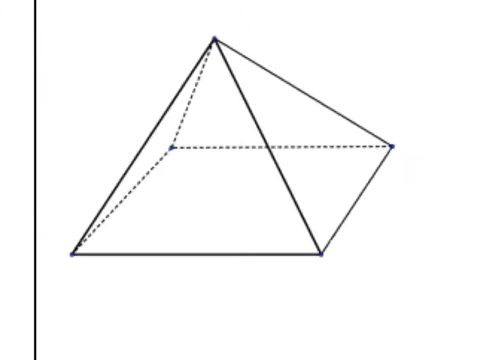 So that I it would create a rectangle. Let me clean this up. Bam, that's going to give us a nice rectangle up in here. What about a square based right pyramid? let's cut. make cuts parallel to the base on this one. so if this is my shape, if I was going to cut parallel to the base and I would need to place my 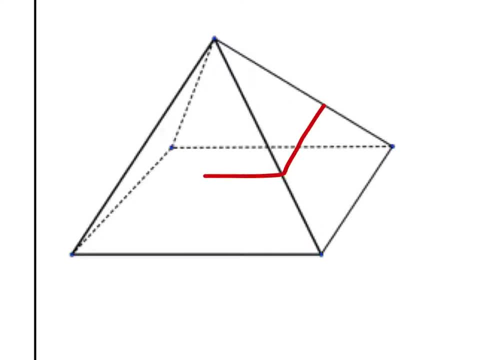 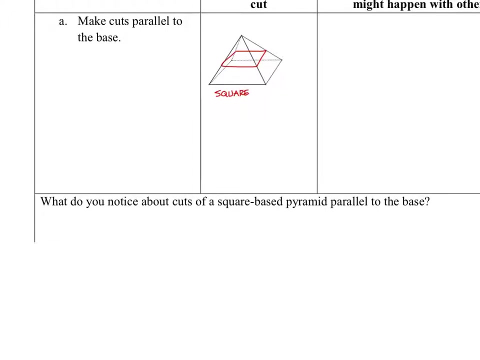 razor blade, maybe right here, and then cut straight back. So what would I get by cutting this straight back? Yeah, this is going to be a square that didn't come out very good, but it is a square. So what do we notice about cuts of a square based pyramid parallel to the base? they are all squares. 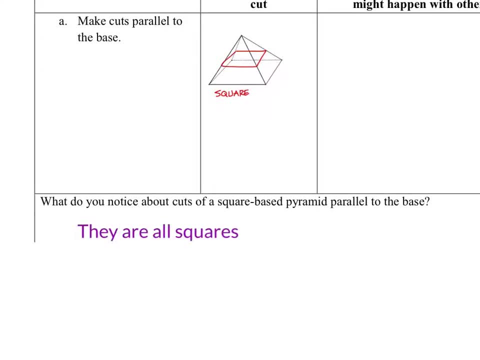 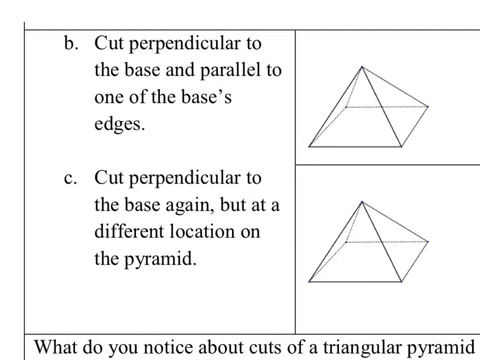 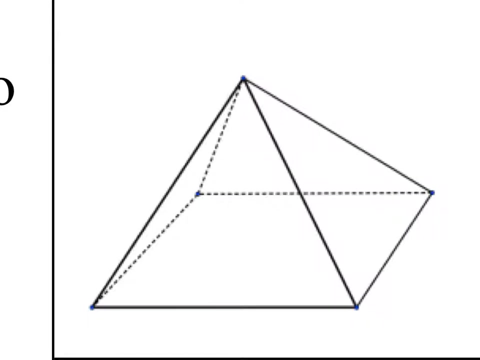 So what do we notice about cuts of a square based pyramid parallel to the base? they are all squares, All right. if we cut this perpendicular to the base and parallel to one of the bases edges, Then then what we get? hmm, So what that means on this is that it would be like starting at the bottom, placing my razor blade. 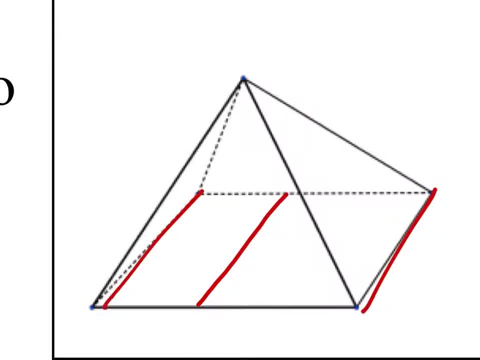 Parallel to the edges, like this edge and this one, and then maybe I was to cut straight up. Well, if I did that right in the middle, I get this triangle right account, But if I move the blade anywhere to the side Then it's going to cut up into this. 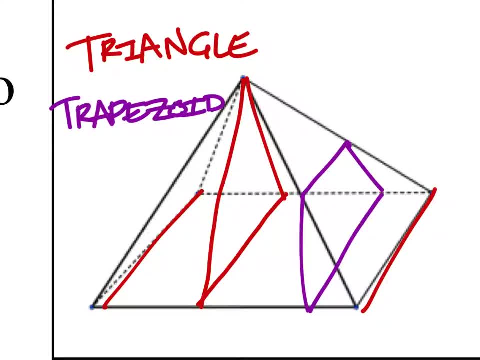 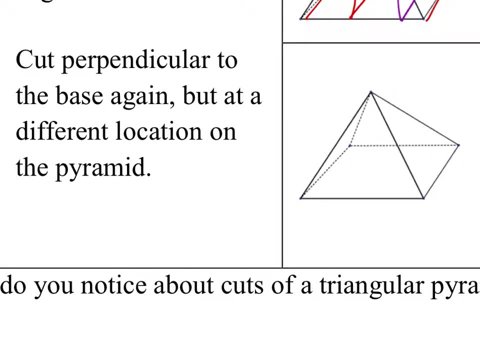 Right account, which makes a trapezoid Just like that. So we'll either get a triangular trapezoid with this type of cut. Next let's cut this perpendicular to the base again, But at a different location On the pyramid. we already did that. That created either a triangle or a trapezoid, depending on which one we're looking at. 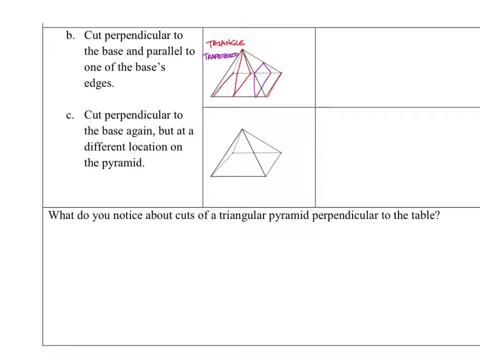 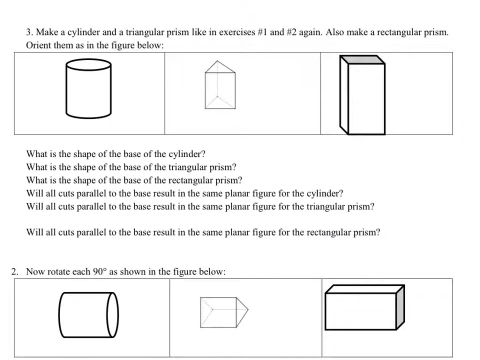 So what do we notice about cuts of a triangle perpendicular to the table? You'll either get a triangle of trapezoid with those. you So on these ones, make a cylinder in a triangle prism- We just looked at those. make it a rectangular prism. orient them like these. that's good. 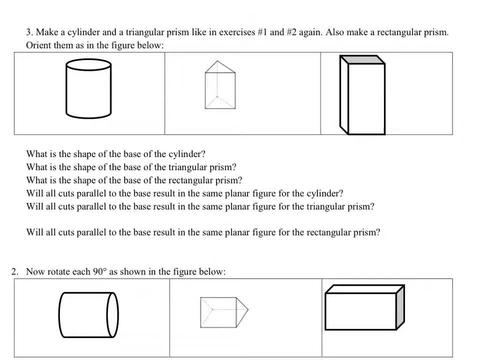 What is the shape of the base of the cylinder? that appears to be a circle to me. What is the shape of the base of the triangular prism? a triangle. What is the shape of the base of the rectangular prism- a rectangle. We'll all cuts parallel to the base result in the same planar figure for the cylinder. Yes, 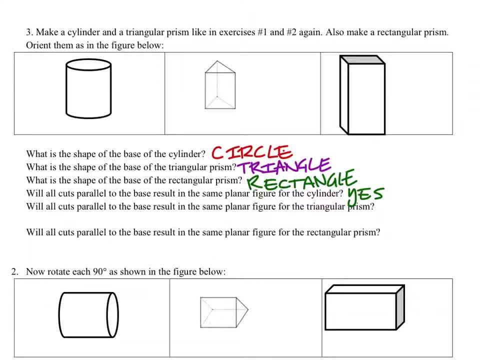 Will all cuts parallel to the base result in the same planar figure for the triangular prism? Yes, Will all cuts parallel to the base result in the same planar figure for the rectangular prism? Yes, Rotate each of these 90 degrees, meaning we're just going to set each of them on their sides. 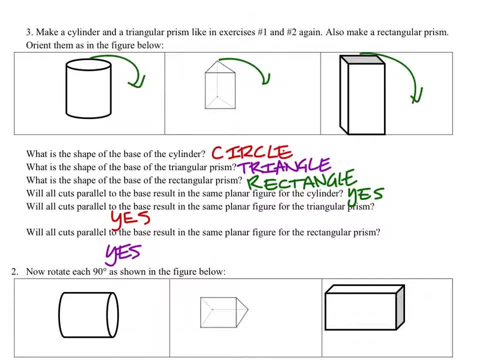 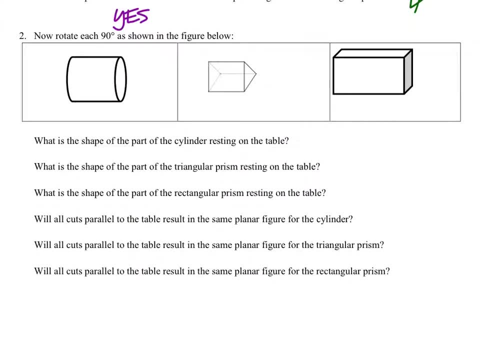 this way, like in the figure shown down here. So now, what is the shape of the part of the cylinder resting on the table? I would just call that a line. You could say it's a rectangle. perhaps What is the shape of the part of the triangular prism resting on the table? 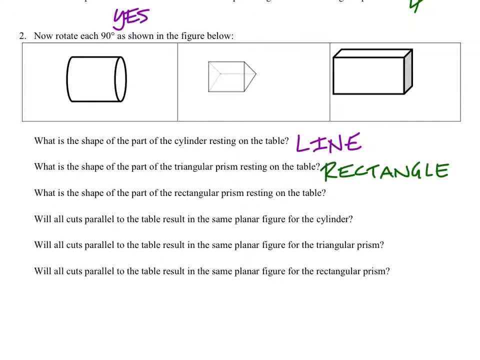 Right now it is a rectangle. What is the shape of the part of the rectangular prism resting on the table? A rectangle? Will all cuts parallel to the table result in the same planar figure for the cylinder? Yes, Do we have any rectangles?